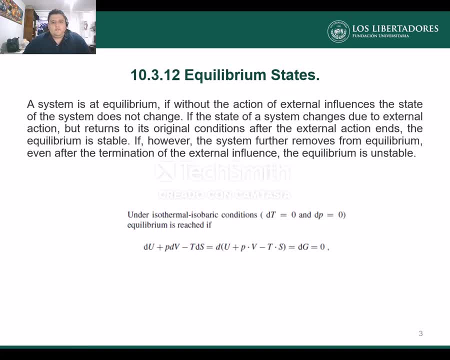 system is equilibrium if, without the action of external influences, the state of the system might change. if the state of system changed due the external action would retold its original conditions. after the external action ends, the equilibrium is stable. if, however, the system father removes for equilibrium even after the termination of 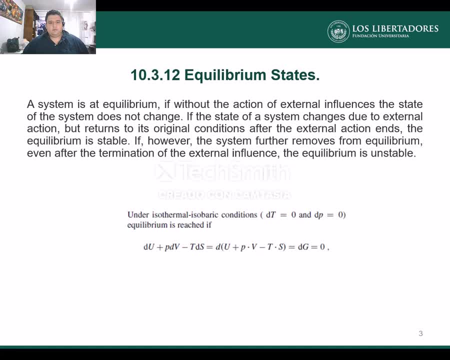 equilibrium terms of certain表 performance. and next, let's conclude to the state of the system, is stable. if, however, the system fathers removes for equilibrium, even after the termination of equilibrium, even after the termination of externally influence the equilibrium, it's unstable. This is the principal. 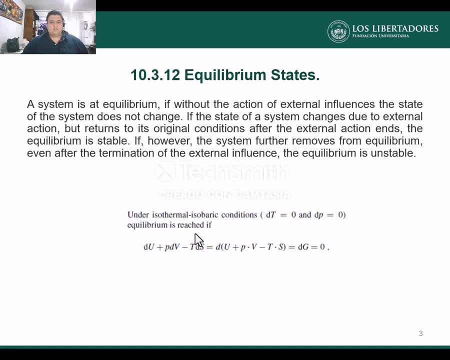 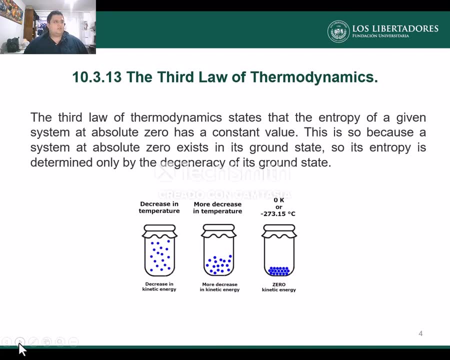 equation for the equilibrium states and thermodynamic application. Next to this, the Dirlau of thermodynamics. The Dirlau of thermodynamics states that entropy of a given system at solid zero has constant value. This is because the system at solid zero exists in the ground states, So its entropy. 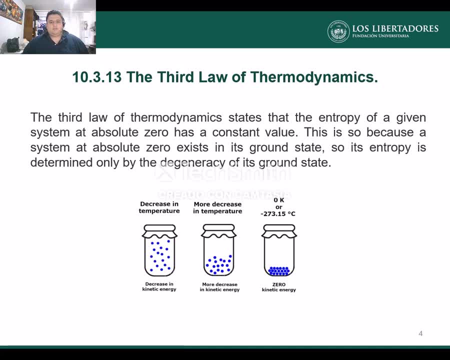 determines only the generality of the ground states And this law determines the generality of the ground states. And this law determines the generality of the ground states And this law completes that the entropy is zero with. because the entropy is zero with. 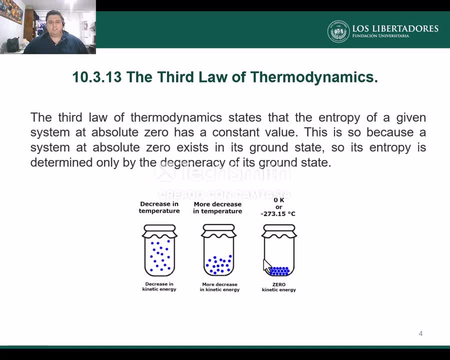 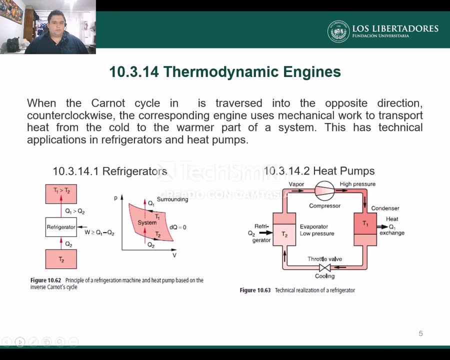 the value zero, Kelvin is reset, With the availability zero, with the temperature zero, the entropy remains constant and does not change. Now the thermodynamic instinct. When the car non-cycles, it travels in an opposite direction, counterclockwise or west side. the corresponding engine uses mechanical work to transport heat for the 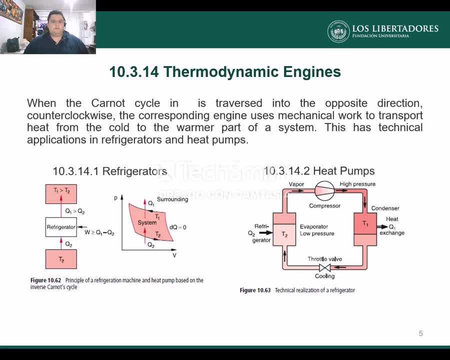 particular part of the system. This is a technical application in the refrigeration, the refrigerator and heat pumps. There are seven main machines in the refrigerator. The refrigerator system is based on a reverse Carnot cycle. The main purpose is its rate heat for the system and lower the temperature. 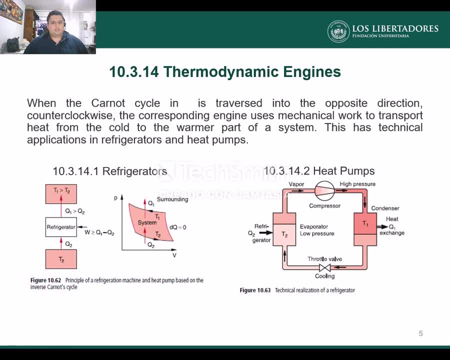 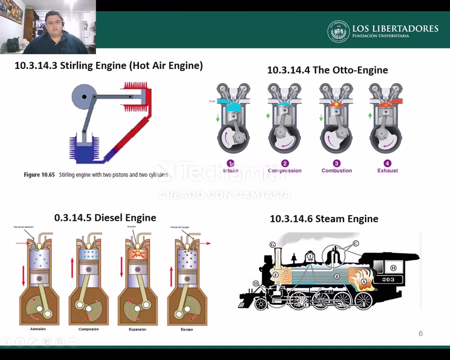 Heat pumps. A heat pump has the purpose of increasing the temperature of a system, with the purpose of using this energy to obtain mechanical work- mechanical energy. The refrigerator system has a helicopters engine. The purpose of the thermotechnical engine is to produce hot air. This can be used, for example, inよう. 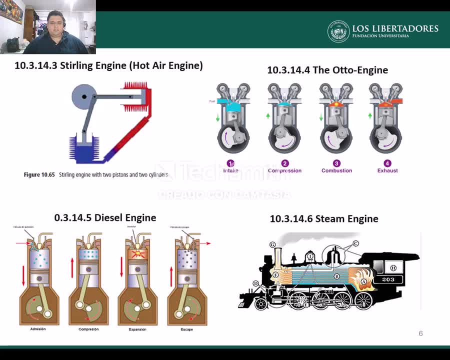 The electric vehicle engine is one of the most widely used engine in the cars, motorcycles and other applications. It is based on four times or four strokes: intake, compression, combust and exhaust. The diesel engine works the compression of air-fuel mixture. this produces an explosion. 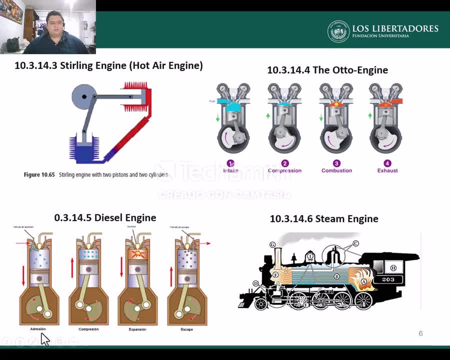 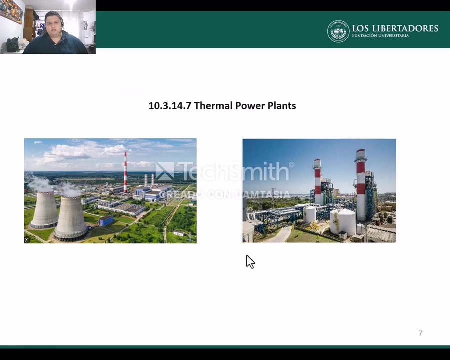 in four times: compression, admission, expansion and exhaust and steam engine. The steam engine is, for example, in the locomotive and thermal power plants. Finally, electric power plants are responsible for providing electricity to homes, to industries. You can find nuclear power plants in some countries.